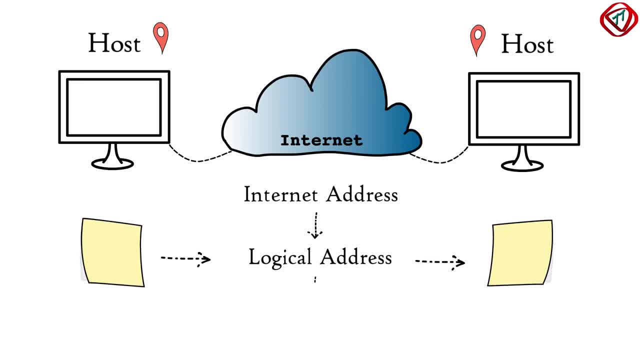 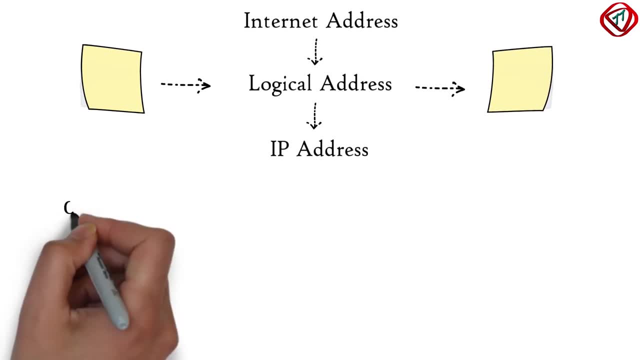 as logical addresses In the network layer. these logical addresses are called IP addresses. If we write a series of binary bits, say 010,, 010,, 01, 11,, we say it is 10-bit in length. Similarly, IP addresses can be 32 bit in length or 128 bit in length. 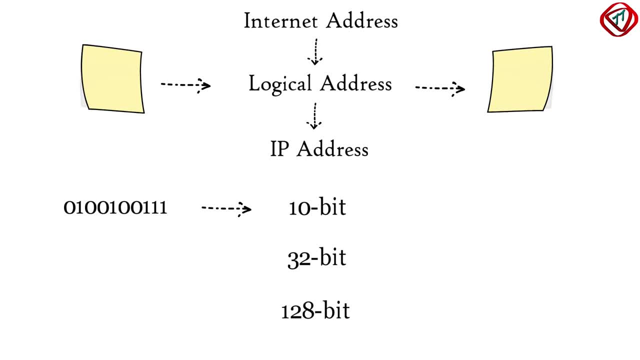 32-bit IP addresses are called Internet Protocol v4 or IPv4 addresses and provide a maximum of 32 addresses. 128-bit IP addresses are called Internet Protocol v6 or IPv6 addresses and provide a maximum of 128 addresses. So IPv6 gives much more flexibility in IP address allocation in a packet-switched computer. 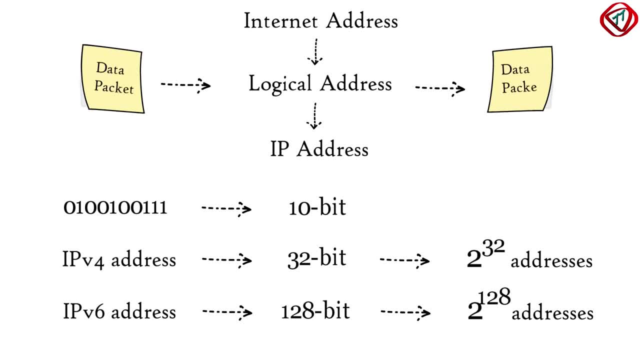 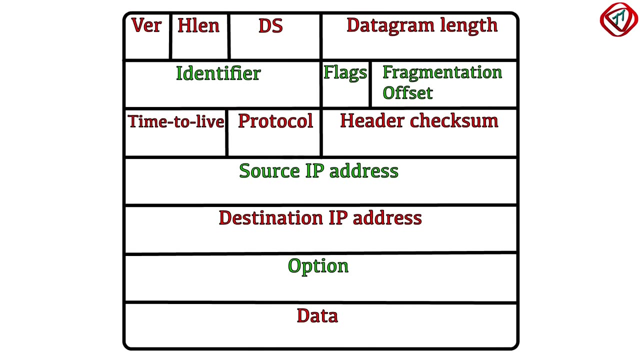 network. Please note that the data packets in the network layer are called datagrams, Based on the version of Internet Protocol used. there are two types of datagrams: IPv4 datagram and IPv6 datagram. Let's understand the format of IPv4 datagram in detail. 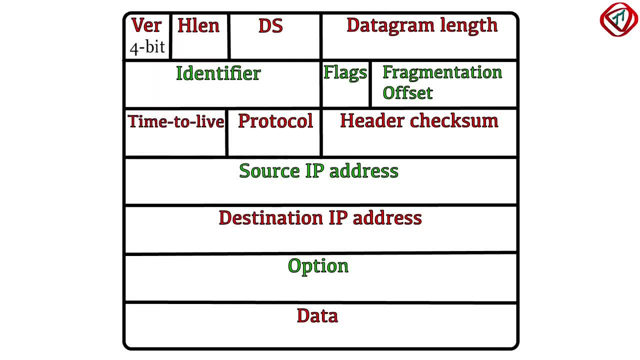 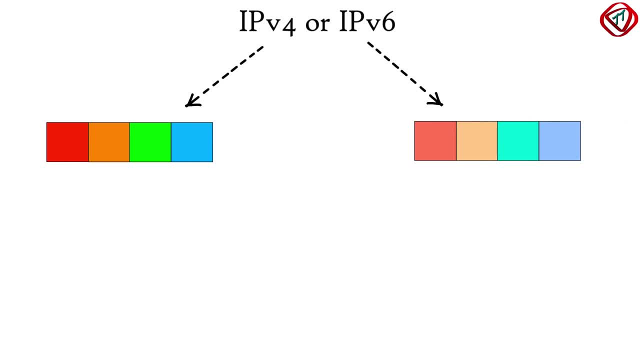 Version number is 4-bit in length And specifies whether the datagram is of version 4 or of version 6.. Different versions use different datagram formats, So this field helps the Internet Protocol software running on a machine to decide how to process the received datagram. 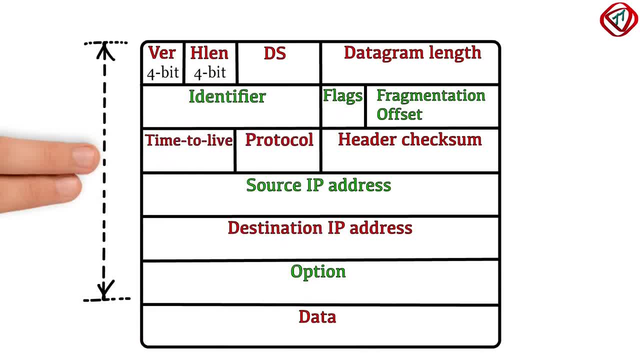 The header length is 4-bit in length And it tells the total length of IPv4 datagram header in terms of 4-byte word, If I say The value in this field is 5. It refers that the length of IPv4 header is 5 words. 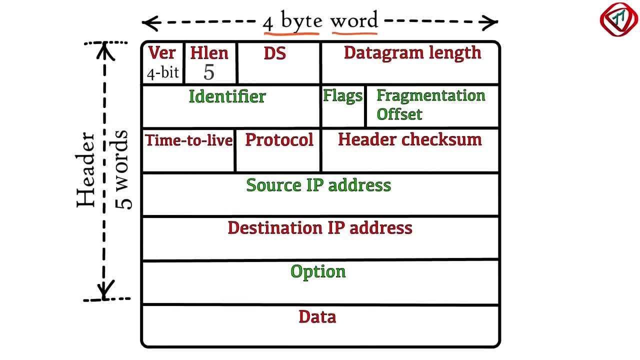 One word in IPv4 is 4-byte in length. Therefore the total length of IPv4 header will be 5 x 4. That is 20 bytes. The option field is variable in length. It makes the IPv4 header vary in length too. 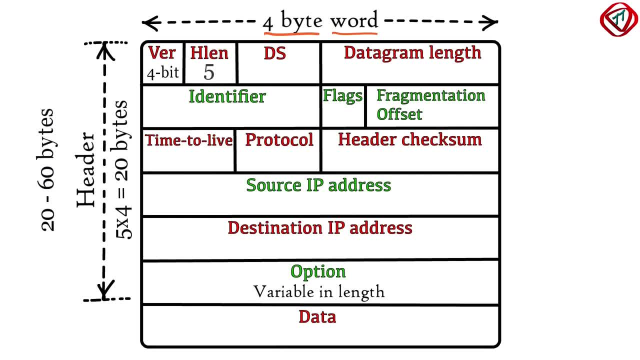 And it ranges from 20 bytes to 60 bytes. The option field is variable in length. It makes the IPv4 header vary in length too, And it ranges from 20 bytes to 60 bytes. If the option field is empty, the value in header length field is 5 or 0101, which makes IPv4 header: 20 bytes in length. If the option field is filled, the value in this field will be 1111 in binary or 15 in decimal format. It increases the header length to 15 x 4. That is 60 bytes. Therefore, IPv4 header varies from 20 bytes to 60 bytes, So the value in header length field is 5 or 0101.. Next to the datagram header is the datagram payload or data. So the value in the header length field indicates where the payload begins in the datagram. 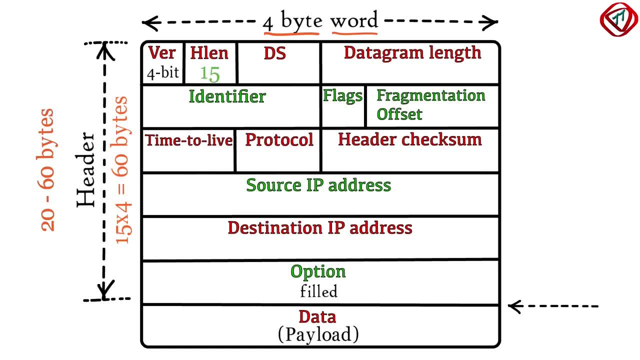 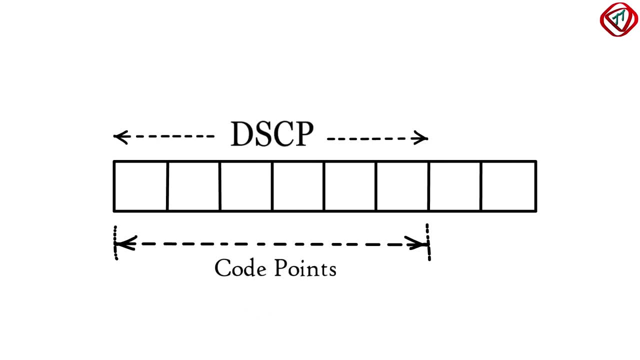 The payload in the IPv4 datagram is transport layers segment. Next is differentiated services. This field is 8-bit in length, out of which the first 6 bits are called code point or differentiated services. code point. Next is differentiated services. First 2 bits in length are called Ihreended And the last 2 bits are used for. you can take. 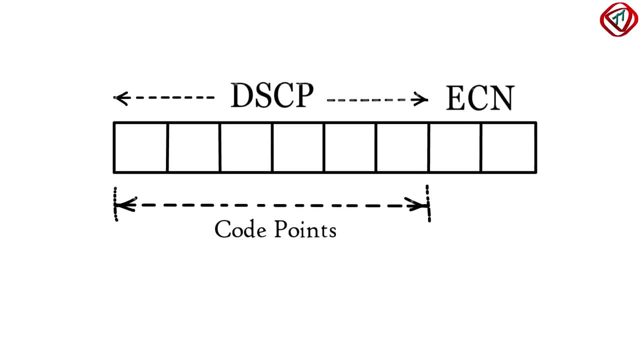 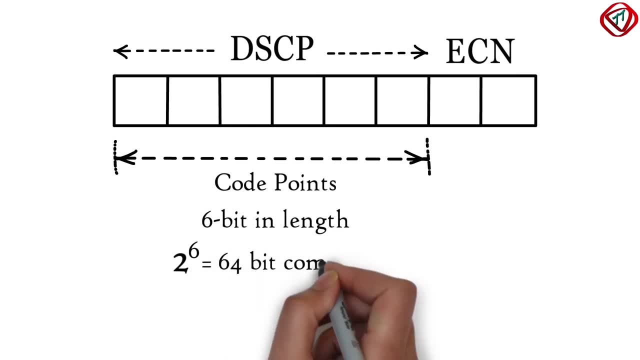 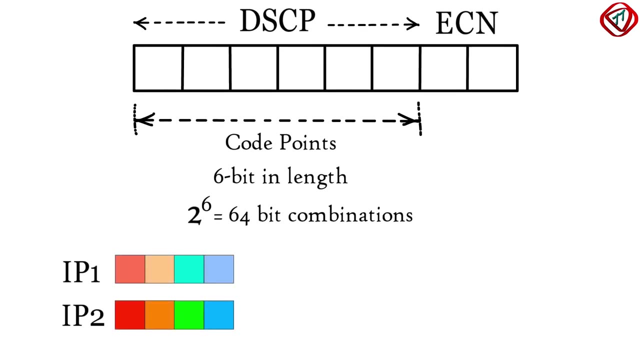 another picture here After Dreward's test: petitonnet check. acious use is angels of gentitution. These bit combinations are used to classify IP packets so that one class of IP packet can receive precedence over the other in a network. For example, IP packet used for network management must get precedence at N. 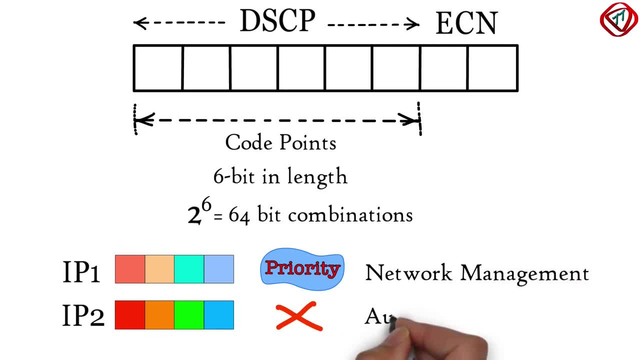 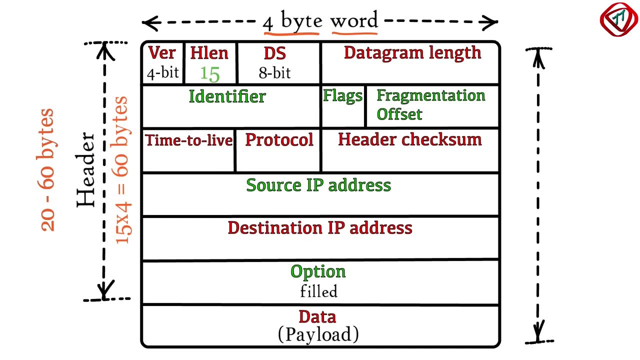 A network power cell- это one of A geh residence- for the transmission over any other type of IP packet. Datagram length tells the total length of the IP datagram, ie header plus data, Since it is 16-bit in length. so theoretically the maximum length of the datagram is 2 raised. 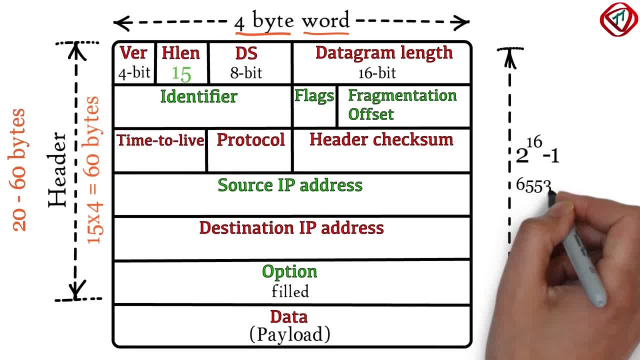 to the power 16 minus 1, or 65535 bytes. however, it is rarely larger than 1500 bytes, which allows the IP datagram to fit in the payload section of the Ethernet frame. The size of the payload field in the Ethernet frame varies from 46 to 1500 bytes. 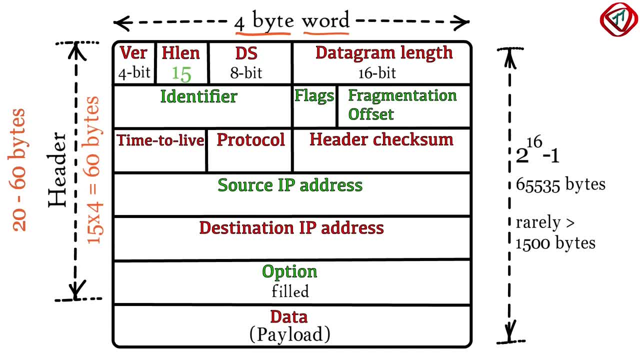 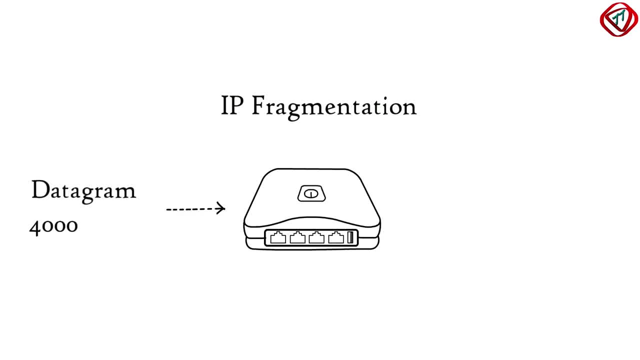 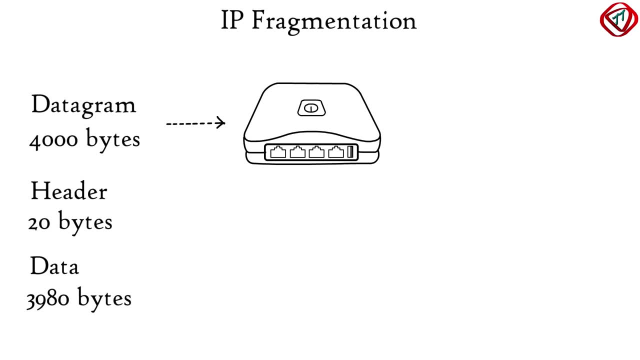 Identifier flags and fragmentation offset are used in case of IP fragmentation. Suppose the router receives a datagram of 4000 bytes. It has a 20-byte header, So data is 3980 bytes. This data should be encapsulated in an Ethernet frame which supports a maximum of 1500 bytes. 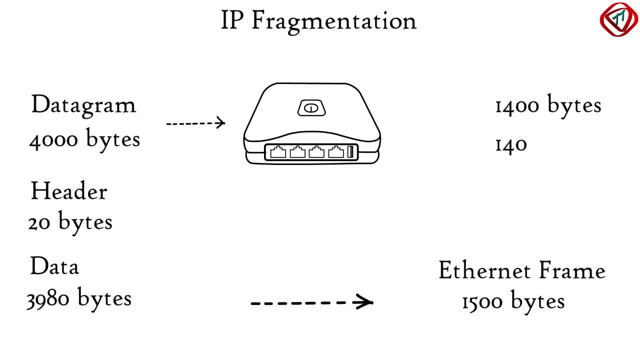 In such a case, 3980 bytes are divided into small units and packed into separate IP datagrams so that the whole data can be transmitted. This is called IP fragmentation. In case of fragmented data, the receiver should be able to identify that these are IP fragments. 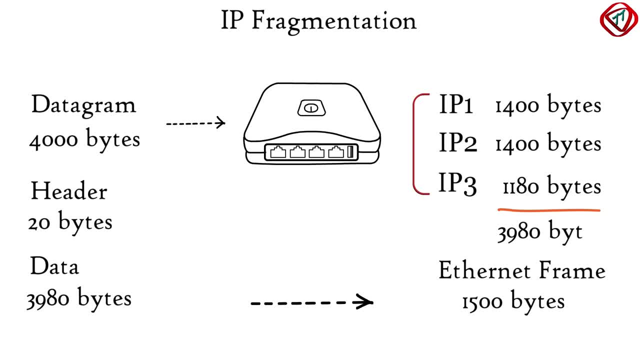 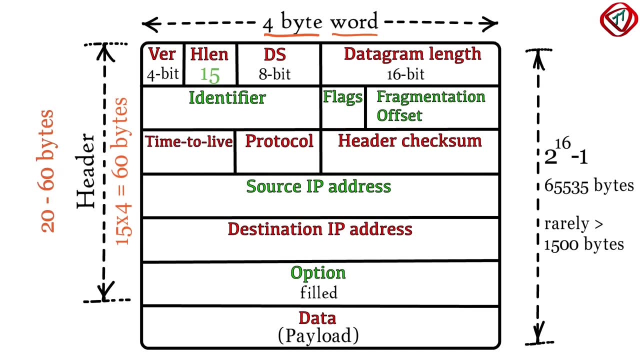 and they should be combined in coordinates. This is the correct order to form the original data unit. Fragmented IP packets are identified with the help of the identifier field. When an IP datagram is created, a value is written in the identifier field. 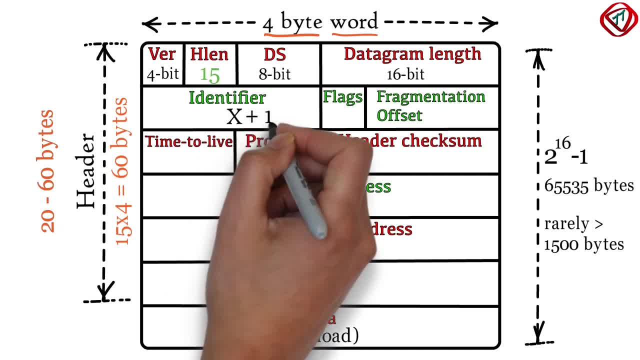 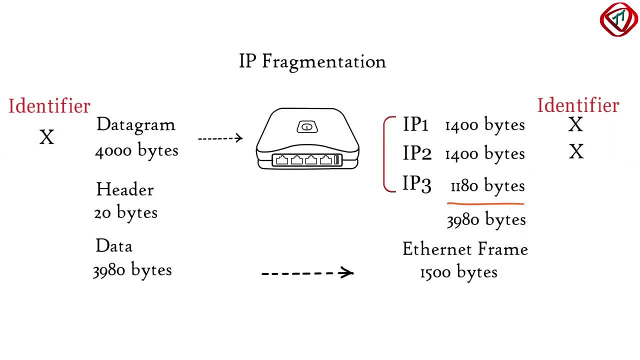 For the next IP datagram, the value is incremented by 1.. However, if the IP datagram is fragmented, the same identifier value is written in all the fragments. Flags are 3-bit in length. The same value is written in all the fragments. 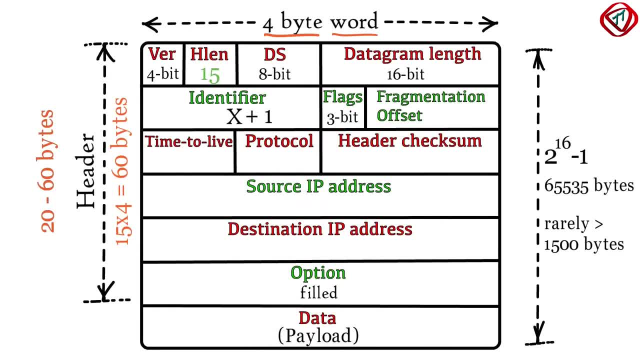 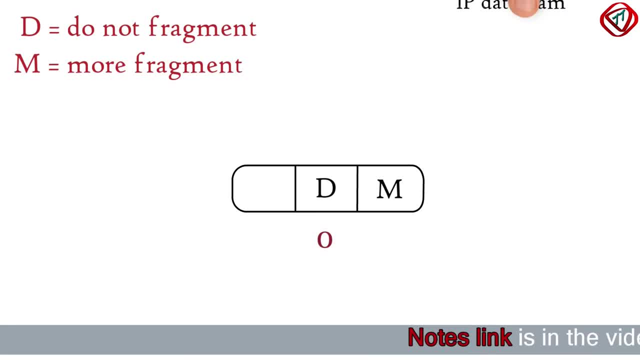 Flags are 3-bit in length, Out of which only 2 bits are used, called Do Not Fragment or More Fragment. If D is set to 0, the IP datagram can be fragmented. If not, it should not be fragmented. 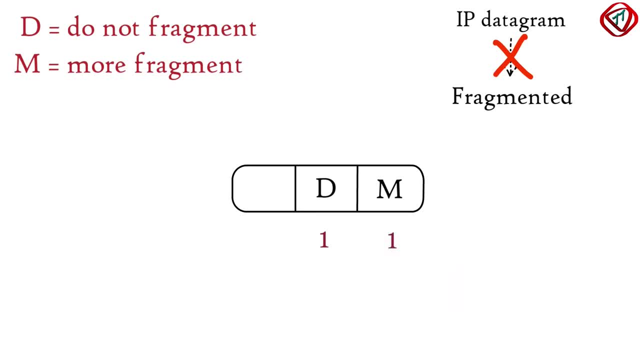 The value of 1 in the M field indicates that the datagram is not the last fragment. If the datagram has 0 in this field, it means either it is the last fragment or it is the only fragment. Now the receiver has identified the IP fragments with the help of Flags and Identifier. 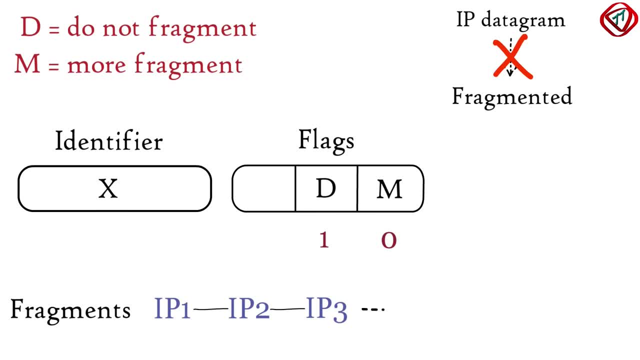 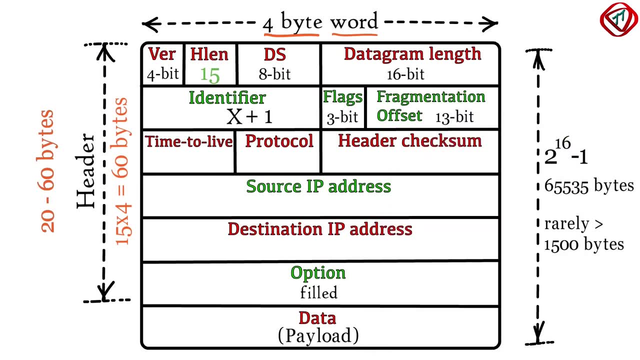 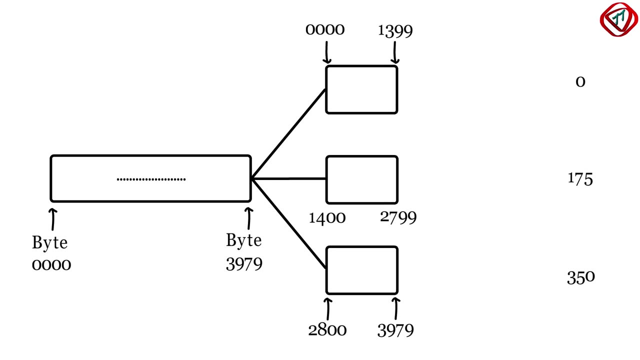 These fragments should be arranged in proper order so as to form the original IP datagram. Here 13-bit fragmentation offset solves the issue. Fragmentation offset tells the relative portion of the fragments with respect to the whole datagram. For the first fragment, the relative position is 0.. 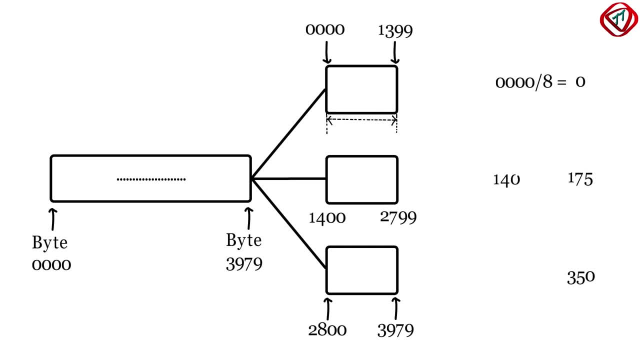 For the second fragment, the relative position is 0.. For the third fragment, the relative position is 0. Adding the length of the first fragment by 8 gives the offset value for the second fragment. Adding the length of the first and second fragment, dividing the sum by 8, gives the. 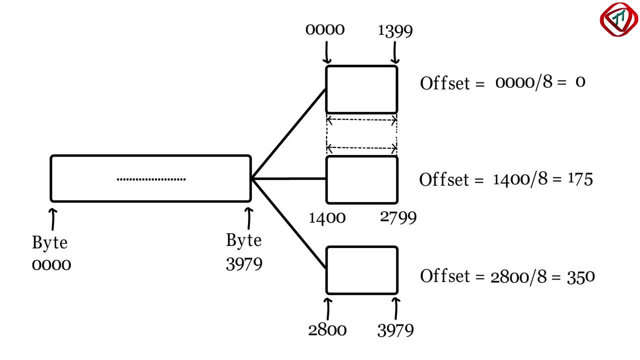 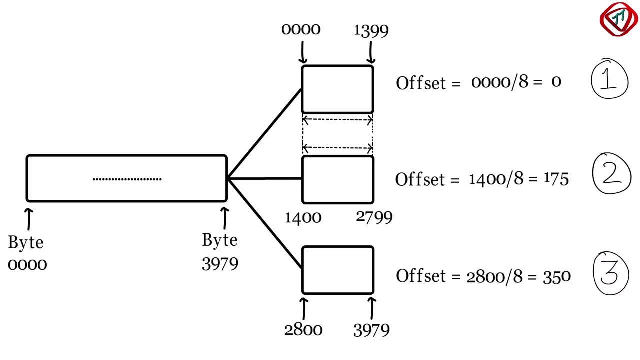 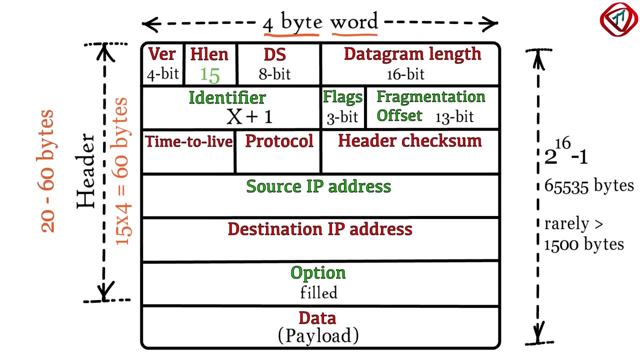 offset value for the third fragment, and so on. In this way, the receiver finds the correct order of the received fragments to form the original IP datagram. IPv6 does not allow datagram fragmentation Time to leave. This field is used to limit the lifetime of an IP datagram as it travels through the 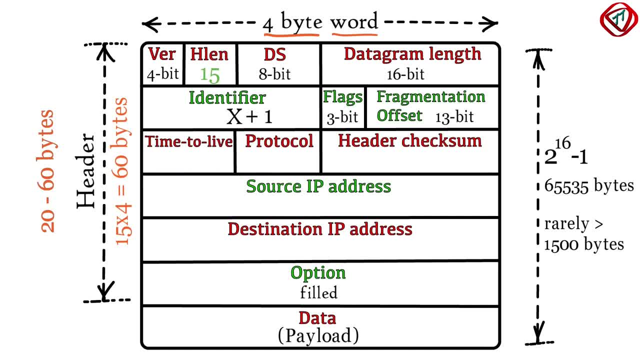 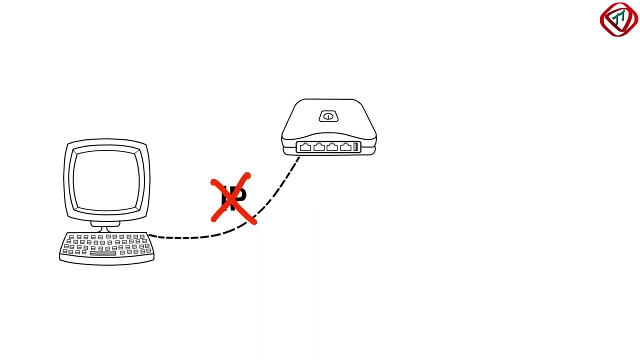 internet. While transmitting a datagram, the source host sets a number in this field. When a router receives the datagram, it decrements this field by 1.. If it reduces to 0, the router discards the datagram, hence limiting its lifetime.